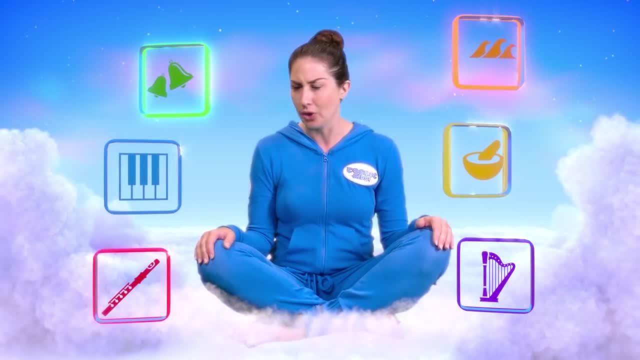 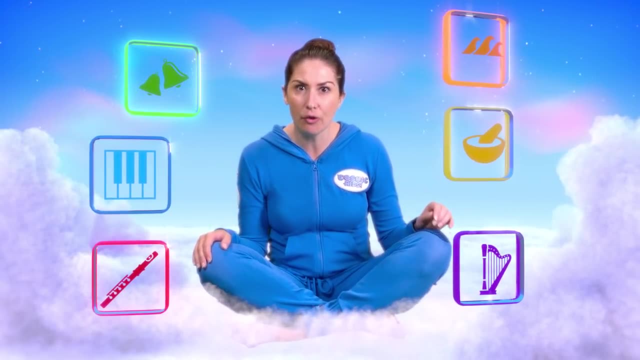 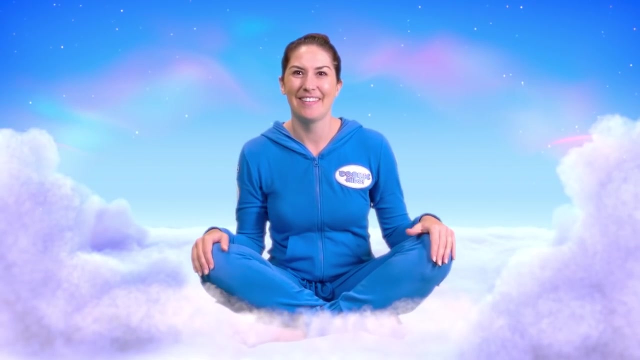 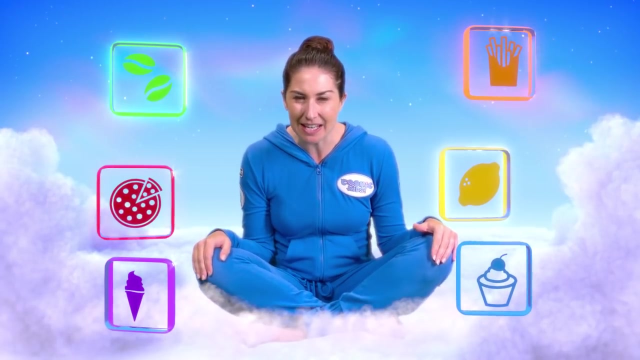 a couple that help us feel all lovely and relaxed. Oh look, a piano tune, Let's have that. Oh, and a soft singing bowl. That's a lovely mix. Now for a smell. Oh wow, look at these, What a fun set of things. Coffee smell- Oh wow, French. 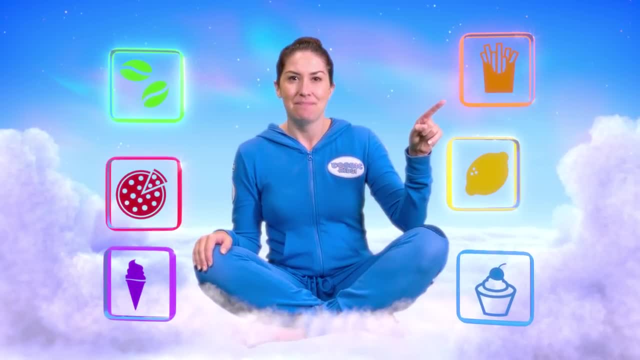 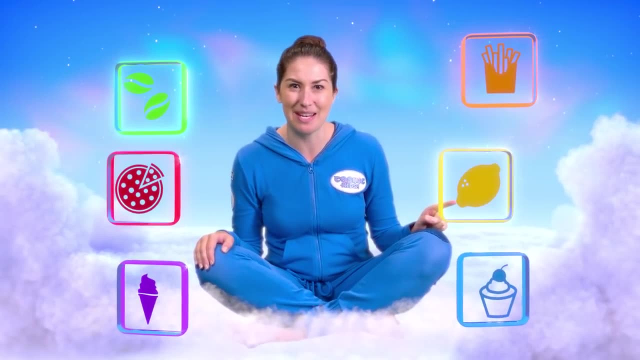 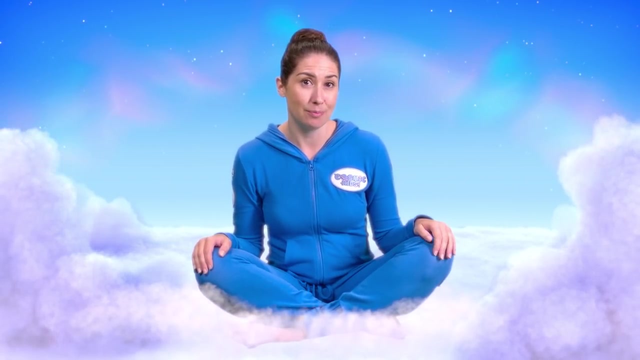 fries, Mmm, that'll make us hungry. Ah yes, let's go for the lemon. That gives us a boost of energy and really wakes us up. Today we're going to talk about the owl and the guard dog- A really interesting way of understanding our brains. But first I'm going to share a 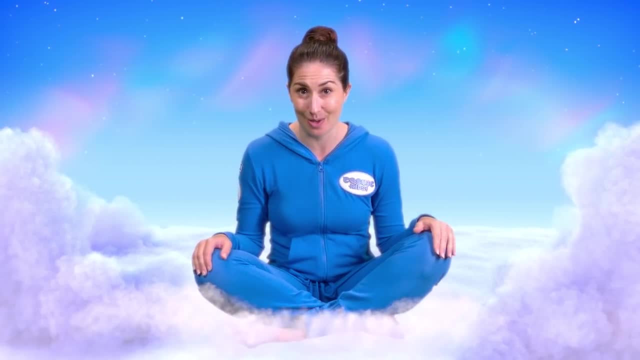 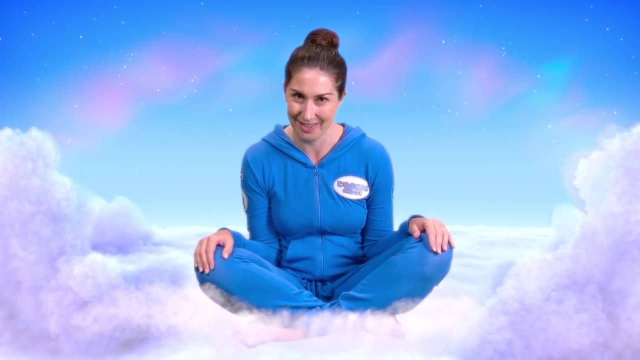 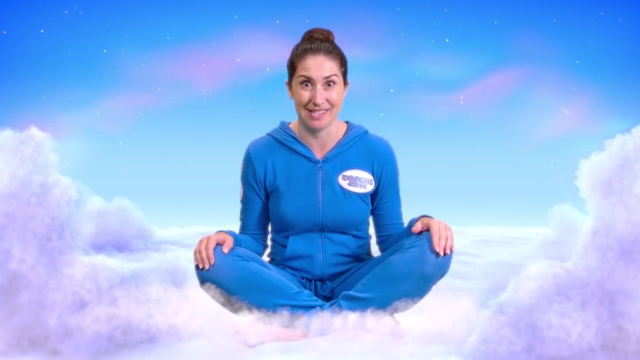 story about something that happened to me when I was eleven years old. At school I was put into the top set for maths. I was very excited because it meant I would be with my friends. I also felt a bit proud that my teachers thought I was clever enough to be in set one. 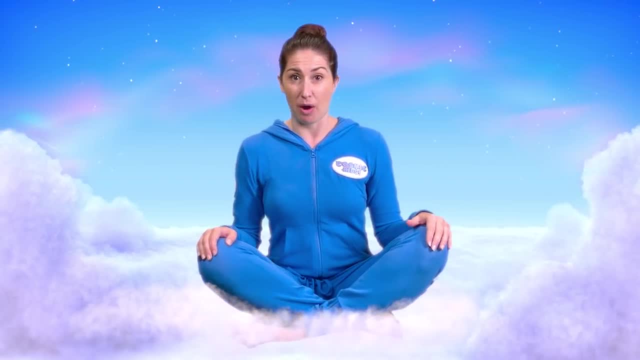 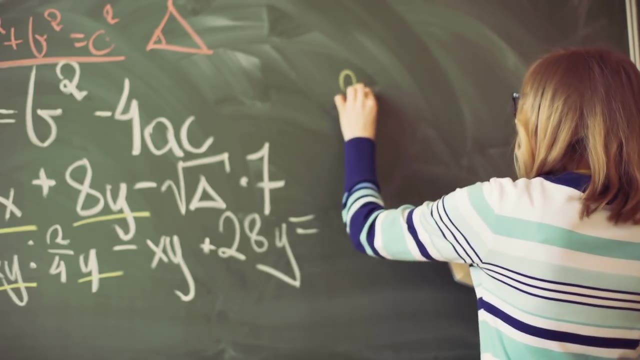 The hardest thing for me in those maths classes was when Mrs Barfield, my teacher, used to write a problem or an equation up on the board. She would just put it up there and then give us a few minutes to work on it. No explanation or anything. 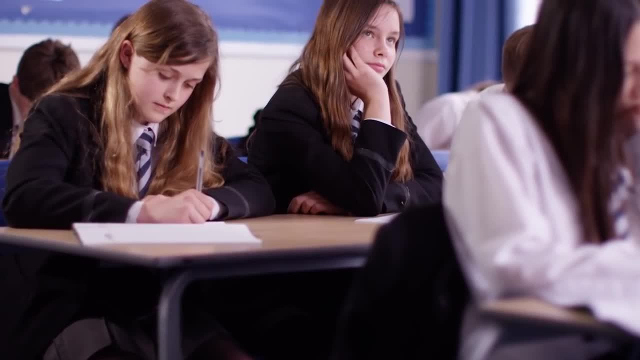 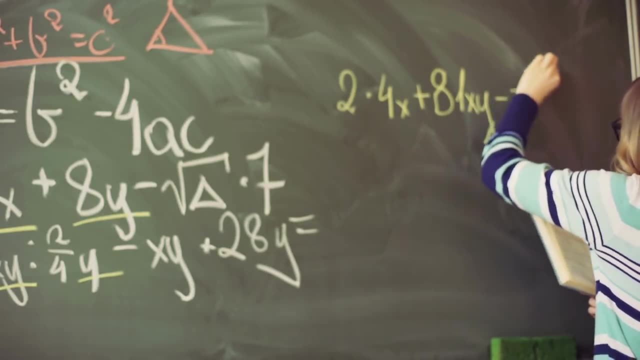 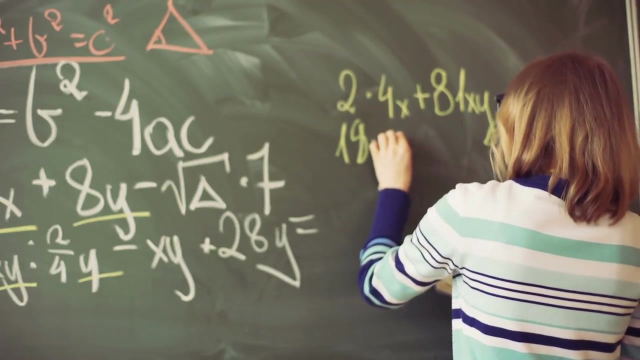 For some reason, whenever she did this, my brain would freeze, I would get into a panic and huff and puff at being made to do it, And I'd even blame Mrs Barfield for being a bad teacher. because I found it so difficult, I once even asked to go to the bathroom just so I could get out of. 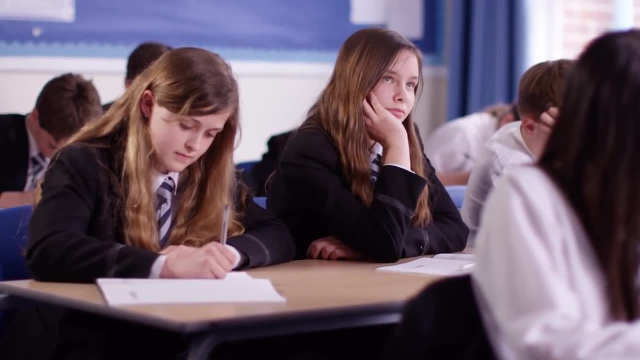 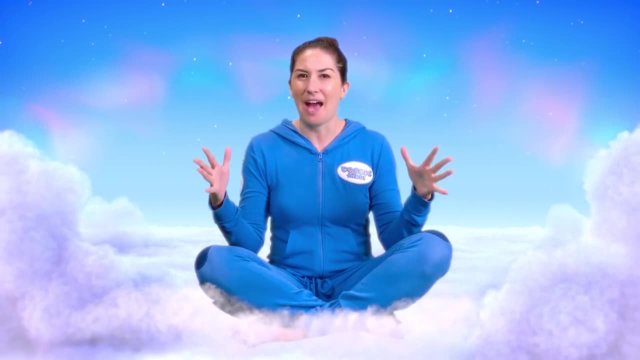 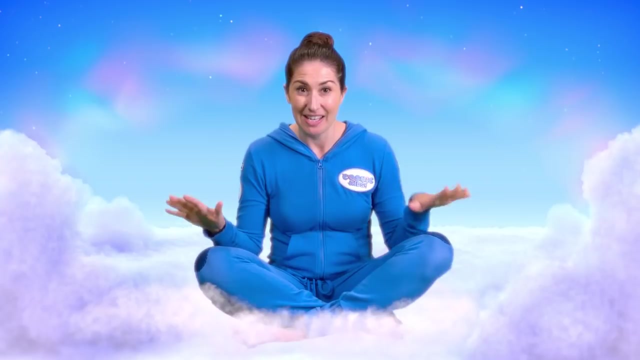 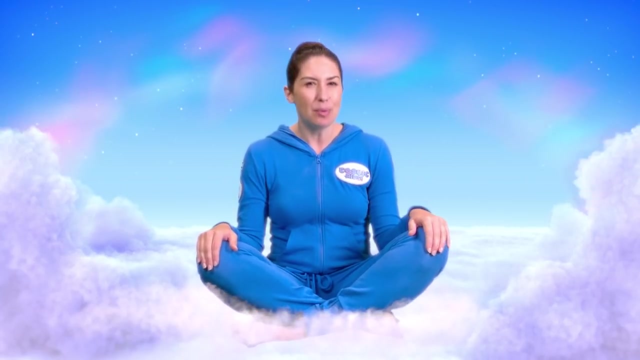 there I got so uptight that I certainly wasn't able to work out the maths problem. Have you ever experienced that Something happens that makes you sort of freeze so you can't even think straight? Well, don't worry, It's quite normal And it's because of how your brain works. You see, our brain is. 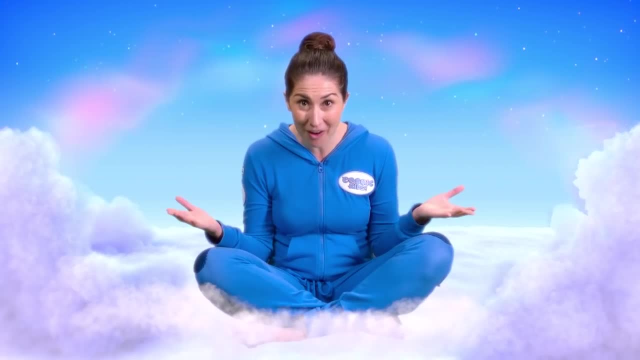 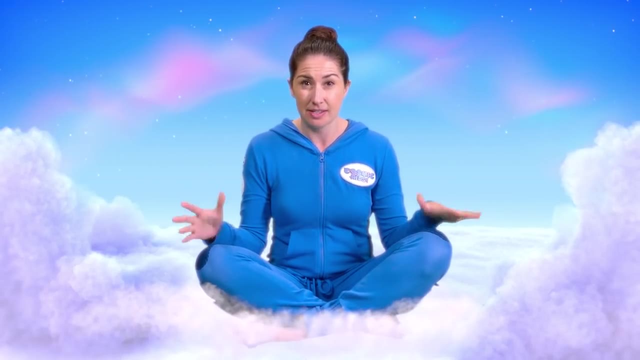 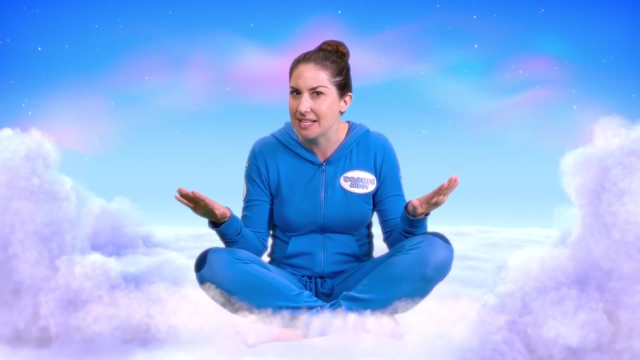 really clever, but above all, it's trying to protect us. It's always on guard in case anything happens that might be dangerous, so that it can help us stay safe of the brain, which sniffs everything out that we're sensing to decide whether it's okay or if. 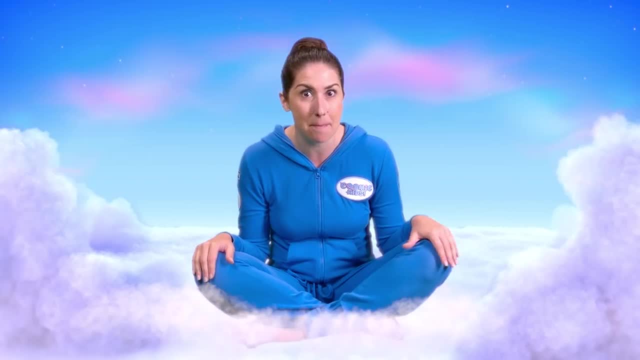 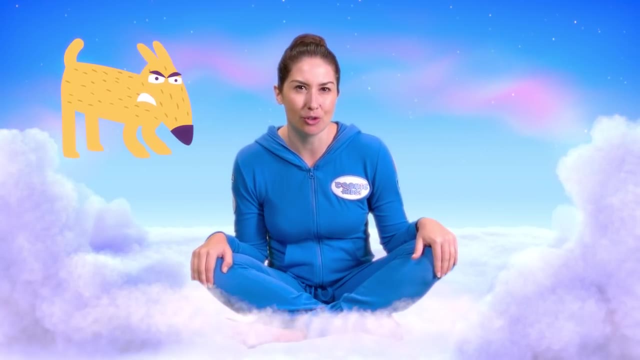 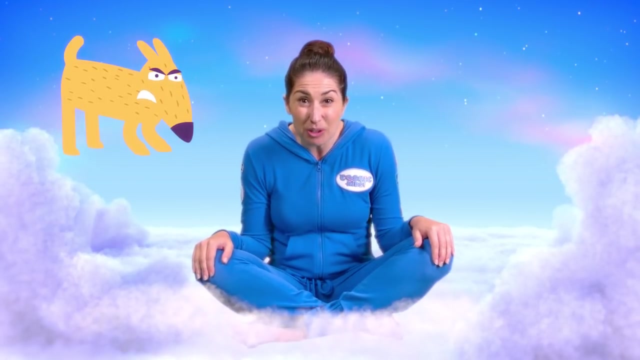 it's a serious threat. it's called the amygdala or, as i like to call it, in your brain, your guard dog. if your guard dog notices something and thinks: hold on a minute, this is scary and dangerous and i don't like it. it'll get your body ready so that you can protect yourself. it gets you ready. 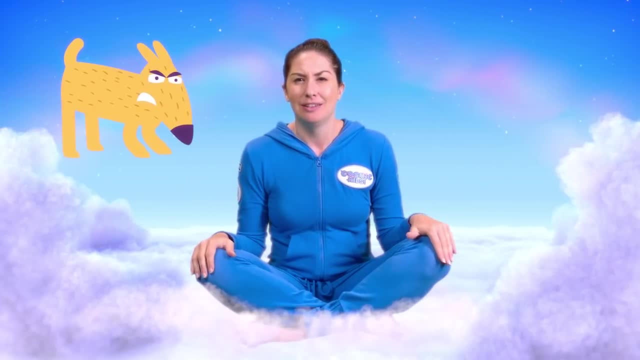 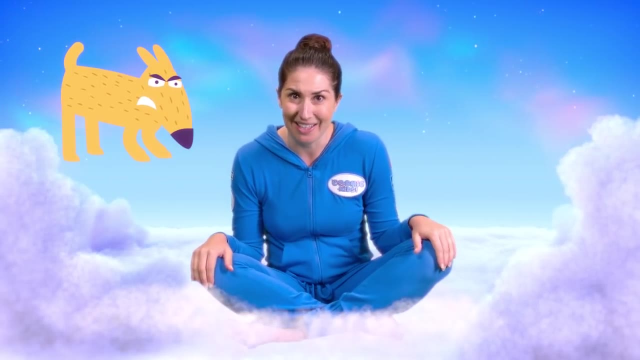 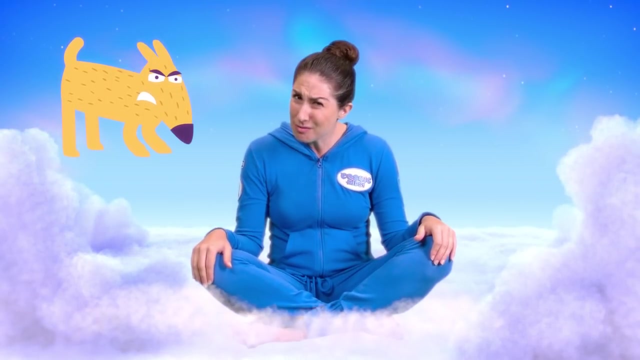 to fight, or it tells you to run away, or it makes you freeze. now, our guard dog doesn't always get it right. it can get carried away, which is what happened in my maths class. the problem mrs barfield wrote on the board wasn't really life-threatening, but my guard dog decided it was, so i froze. i. 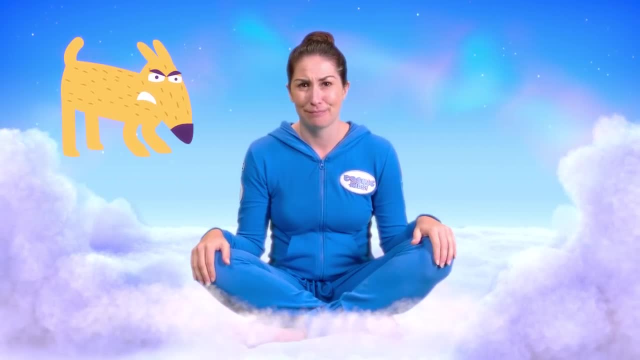 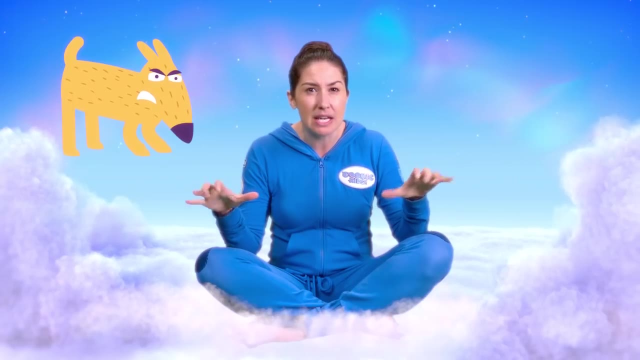 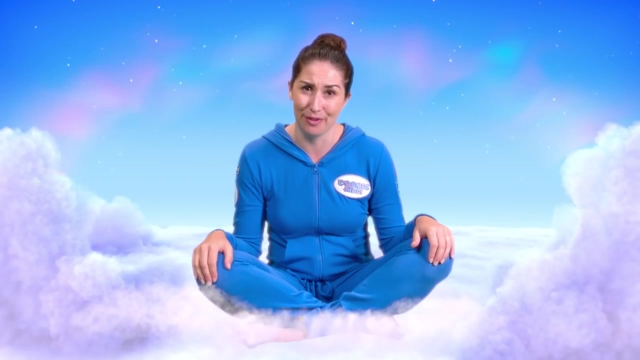 wanted to fight. i even wanted to leave. i felt stupid and embarrassed that i was in a class where i couldn't understand. so the guard dog in my brain started barking loudly and running around protecting me. this makes it impossible for the part of my brain which can. 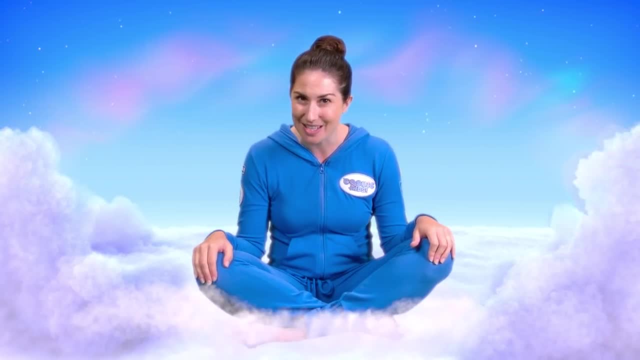 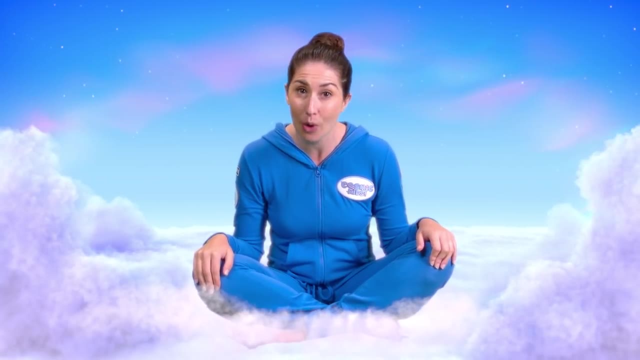 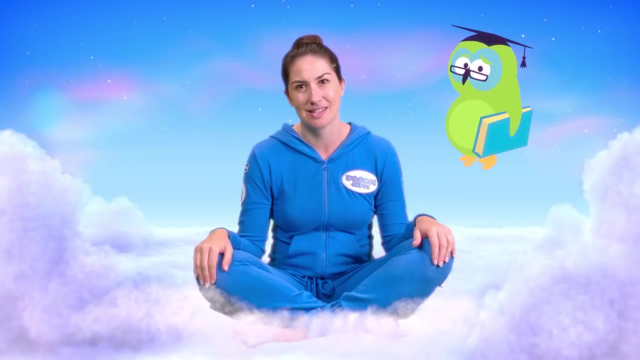 solve maths problems to get involved. this part is called the prefrontal cortex, right up here at the front, or, as i like to call it, your owl. owls are wise, you see. they're thoughtful and good at thinking about things. had i been able to calm my guard dog down, my owl might have had a chance at solving. 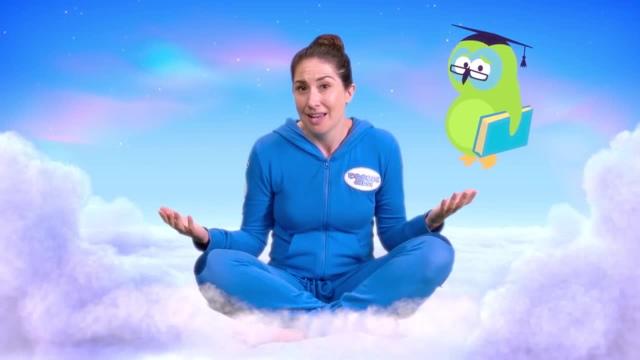 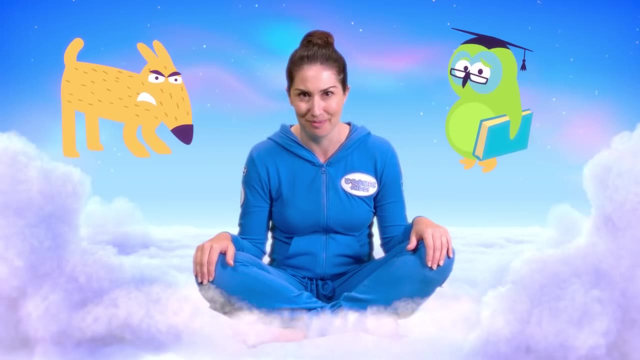 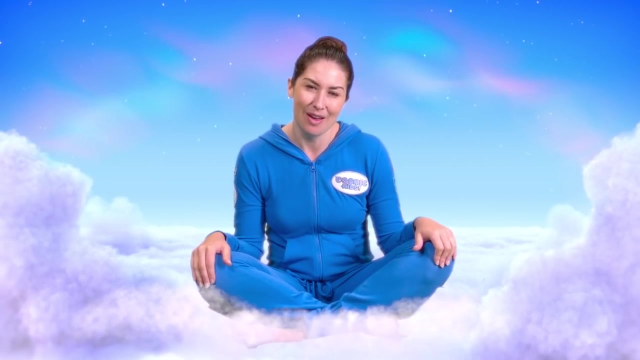 that maths problem, or if it couldn't solve it, it would have shown me how to ask mrs barfield for some help. instead, my guard dog had taken over and was making me panic, so my poor owl didn't get a look in. maybe you can think of a time when your guard dog caused you to react in a way that didn't. 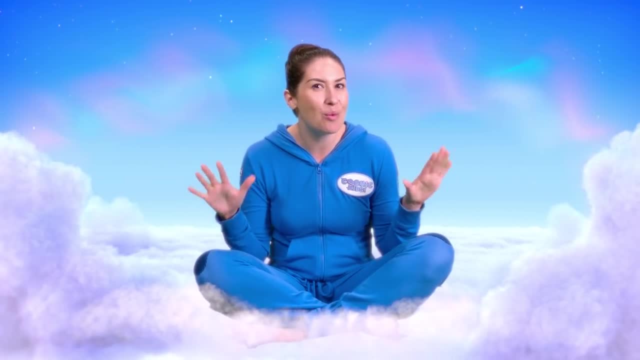 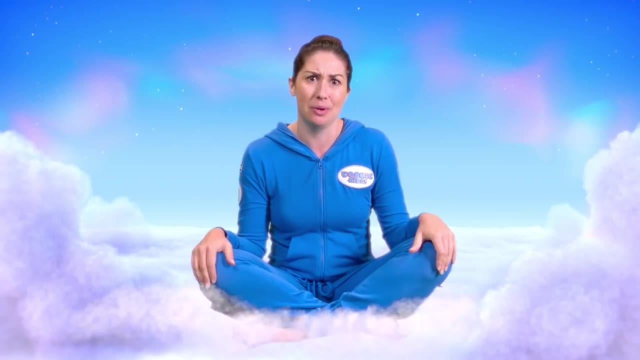 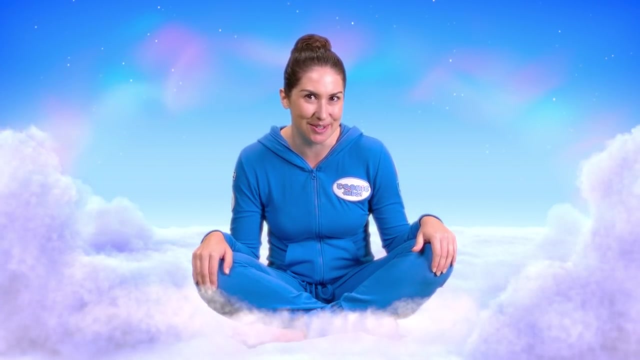 really help you a time when your clever wise owl didn't get the chance to help you out. your guard dog was too busy trying to protect you, even though you didn't really need it to, so you were fighting or freezing or running away. so what can you do about that jumpy guard dog? what would a zen den master do? 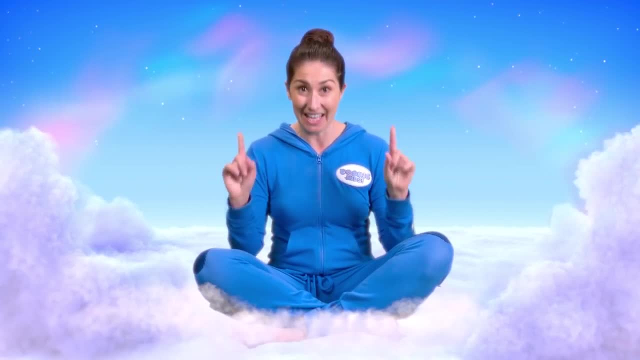 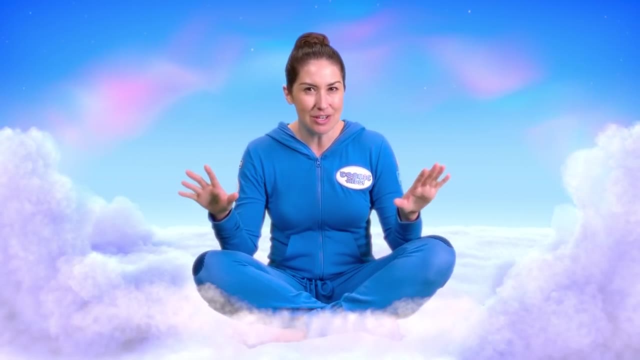 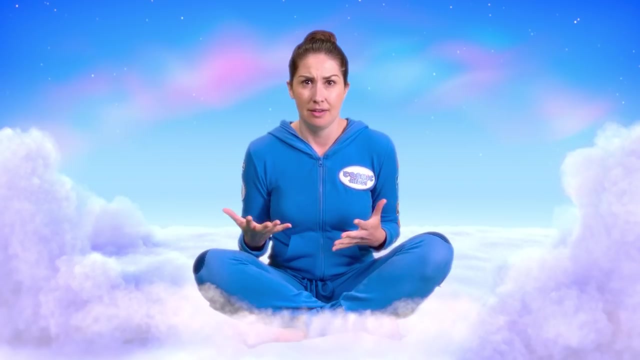 to get it all under control. well, here's something you can try the next time you feel your guard dog taking over. first see if you can just notice him starting to get upset. do you feel yourself want to run away? do you feel the urge to start arguing or fighting, or do you feel like you're frozen to the spot? 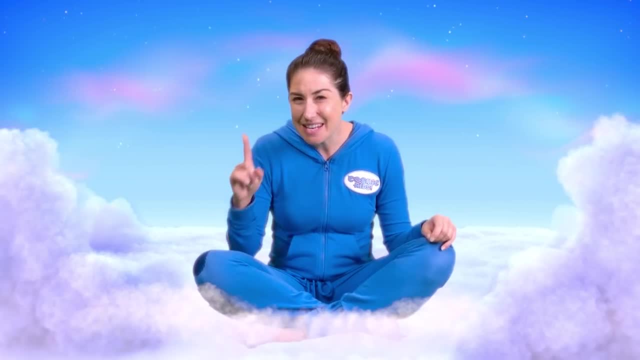 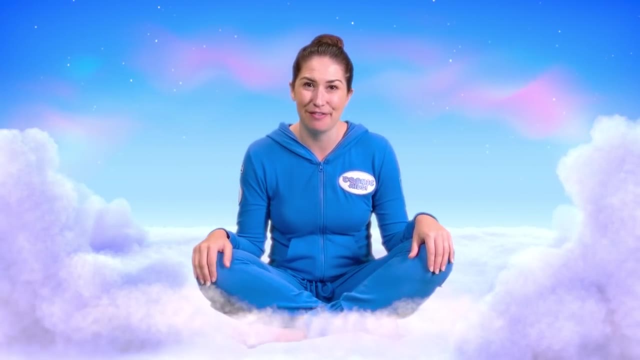 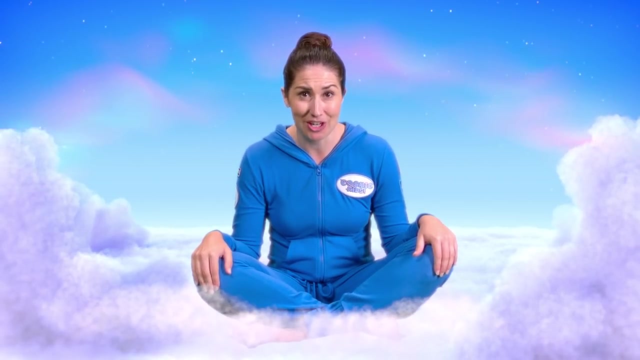 and you don't know what to do. these are the warning signs of it taking over. it happens to all of us. actually, it's trying to keep us safe. the key is: what do you do now? the best tool I know is called The Magic 10. with the Magic ten, you count from ten down to one. 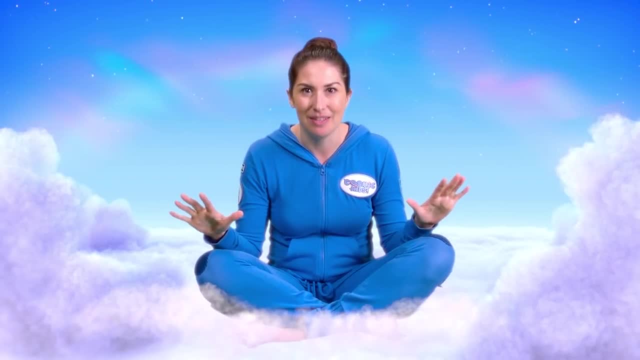 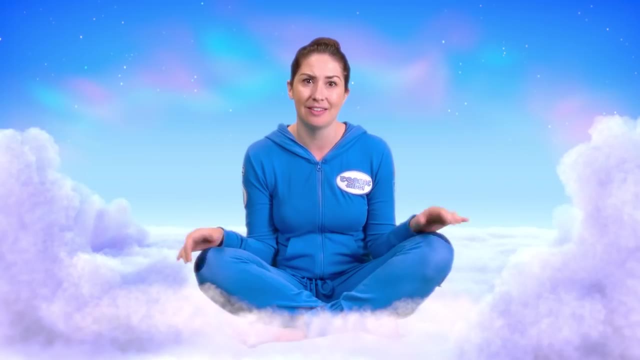 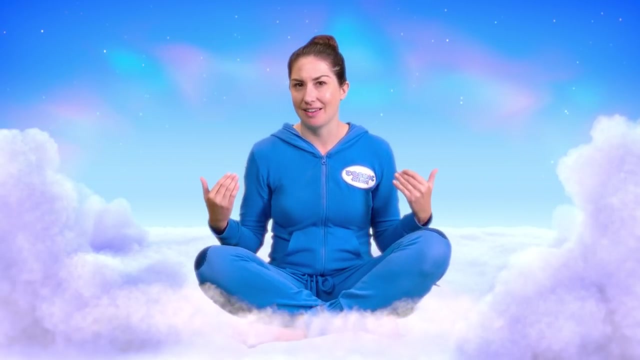 giving your brain some magic time to be calm and process what's going on before you say or do anything, even if you've started to fight already, rather than carrying on, step back and take a magic 10.. Let's see what this does to our guard dog. 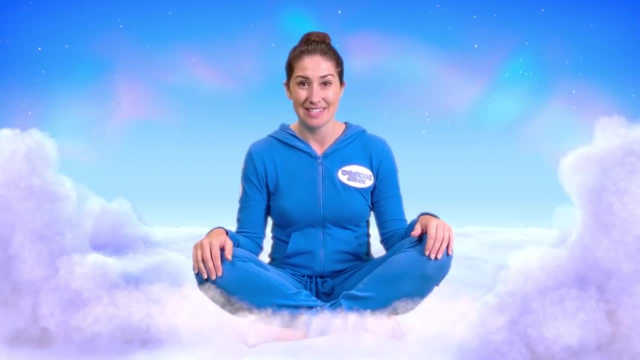 Count with me now from 10.. 10,, 9,, 8,, 7,, 6,, 5,, 4,, 3,, 2,, 1.. There Can you see how he's less worried now He's happier. 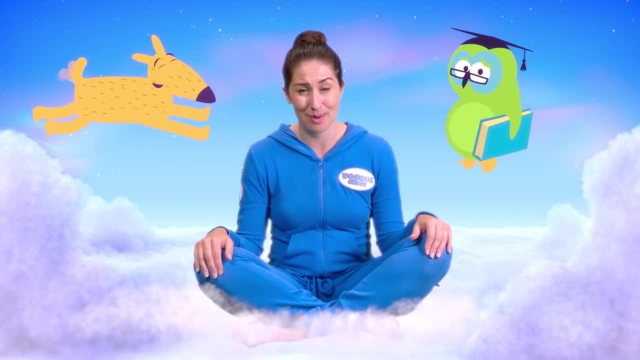 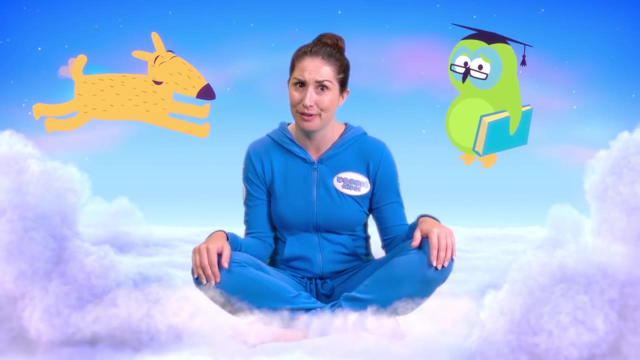 And so our lovely owl can get a chance to help us work out what to do. Of course, your guard dog is very important. He is there to save your life If there is a real threat, like a fire or you get lost. 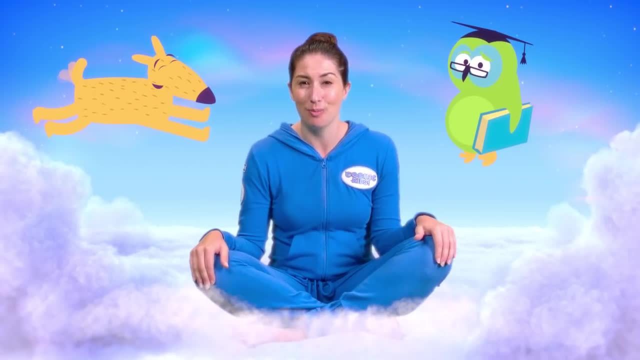 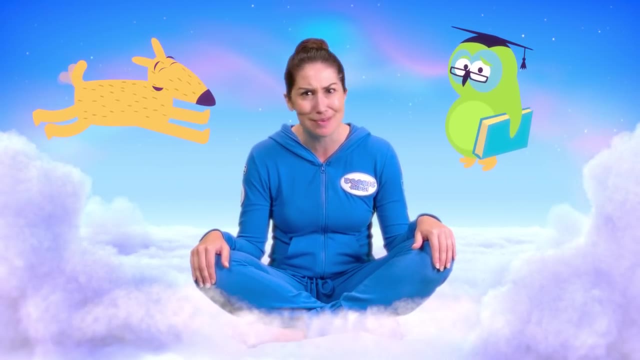 or you need to rescue someone. your guard dog will make sure that you make things happen until you're safe again, But sometimes he can just cause a great deal of trouble. He can make big fuss over nothing. that isn't helpful. It's good to know, isn't it? 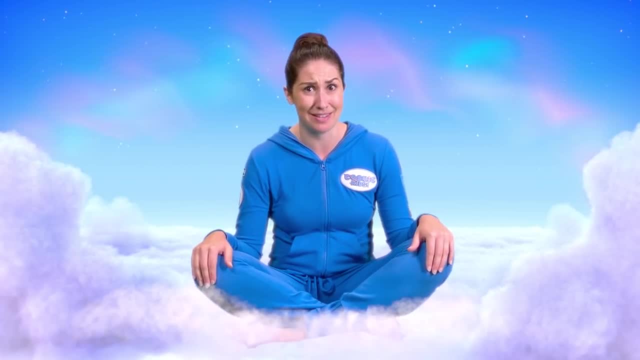 I wish I had known about my guard dog when I was 11 in my maths class. I might have been able to get some help And maths would have been much more fun for me And Mrs Barfield, Hopefully understanding your brain in this way.